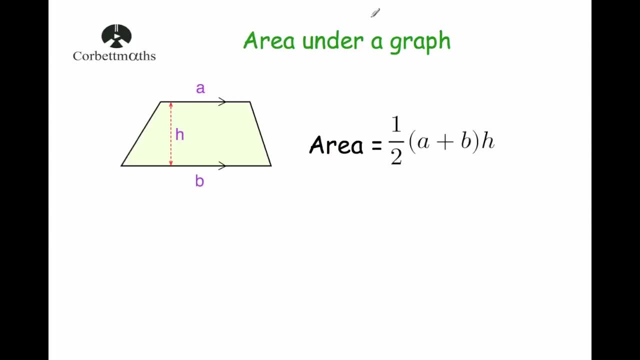 Triangle: half the base times the height and trapezia. I just want to have a look at it quickly. The area for trapezium is half a plus b, which is the two parallel sides added together and then times by the height. So, in other words, to find the area for trapezium, you add together the two parallel sides, half it and times by the height. Now, one thing to note is, whenever we find the area under a graph, quite often these trapezia will be on their side, like: so Okay, and what we'll be doing is we'll be adding together the two parallel sides, which would be the two vertical lines We'll 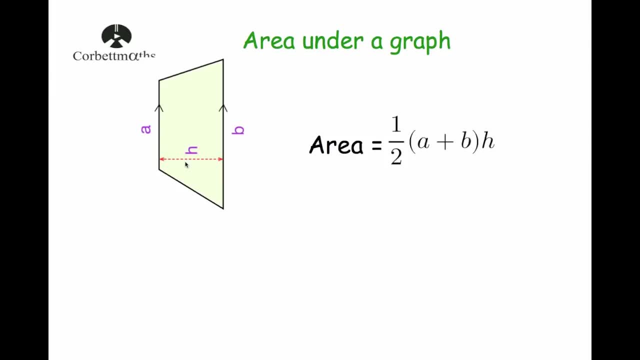 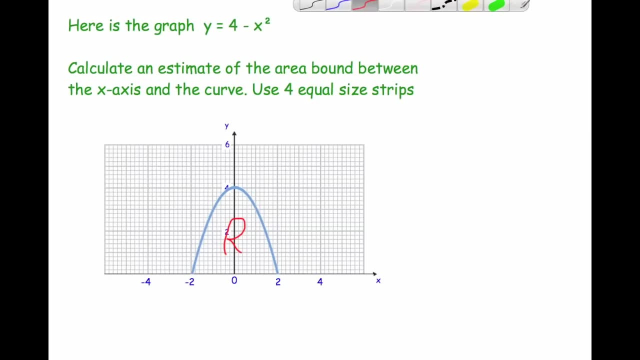 be halving that and then timesing it by the height or the distance between those two parallel lines. Okay, so let's have a look at our first example. Our first example says: here's a graph of y equals four minus x squared, and the question says: calculate an estimate for the area bound between the x-axis and the curve. and I've marked that with the letter r, and we're to use four equal size strips. Now, since the graph goes from minus two to two, well, that's going to go minus two, one zero. sorry, minus two minus one, zero one two. It's going to. 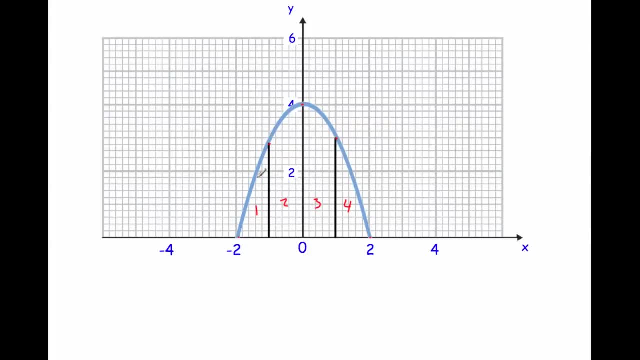 be split quite nicely into four regions. Okay, you've got region one, two, three and four, and I've done that by just drawing vertical lines up at minus one, zero and one- and then you've got the four regions. Now it's quite difficult to find the areas of these regions because this isn't quite a triangle. it's got a curve and obviously this is a curve as well. So what we're actually going to do is we're going to consider them as triangles and trapezia. So here you've got triangle one, trapezium two, trapezium three and triangle four. 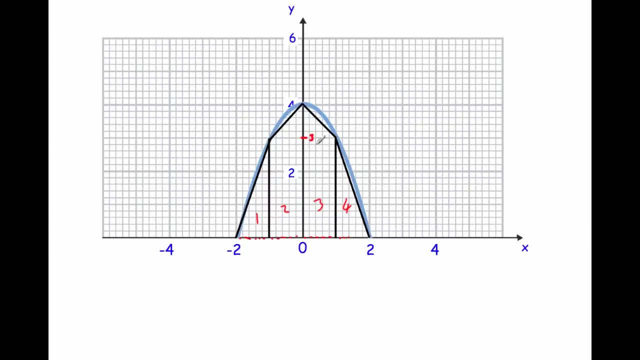 And if we find the areas of these four different shapes, we'll get an area which is pretty close to the area of the whole region. underneath the curve, You see, we're leaving out tiny bits, but this is as close as we can get at GCSE level. So what we're going to do is we're going to find the areas of triangle one, trapezium two, trapezium three and triangle four. Okay, so first of all, let's consider triangle one. Now, just remember that, because the trapezia, that each trapezium has the two parallel sides and we're going to call this. 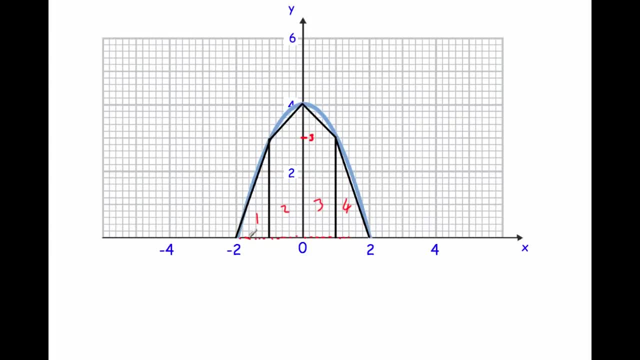 distance between them, the height. I'm going to call this distance of each triangle the height. this distance, the height and this distance the height. I'm going to call that the base and that the base. In other words, I'm going to sort of turn my head sidewards and look at the triangles and work out the area that way. Okay, just so that I'm using the same value for H, the height, for each of the four strips. Okay, so triangle one. So the area of the triangle is half the base times the height. So that's going to be given by a half times the base. Well, the base is going to be this length here, which is three times the height. 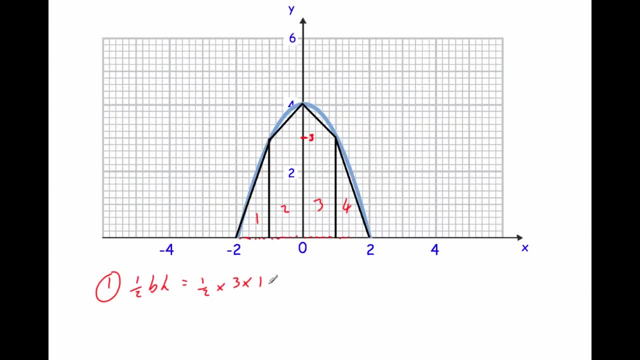 Well, that's the height of the triangle there, which is one A half times three times, one will give us 1.5.. Trapezium two now. So to find the area of trapezium two, we're going to use the formula half bracket, A plus B times height, or the distance between the two parallel sides. So we're going to do a half bracket, Well, the two parallel sides. well, this one has a length of three and this one's got a length of four, So it's going to be three plus four, and then we're going to 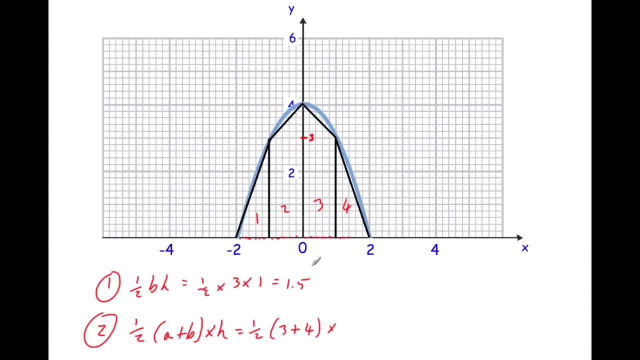 times it by the distance between the two parallel sides, which is one. So we're going to do that. So three plus four is seven. Half of that, 3.5 times one, is 3.5.. Now, interestingly, this curve has got a line of symmetry, that is the y-axis. So the area of two will be the same as area of three and the area of one will be the same as area of four. I'm just going to work out the areas just to show you anyway. Okay, so three To find the area of the trapezium. again, it's going to be half. 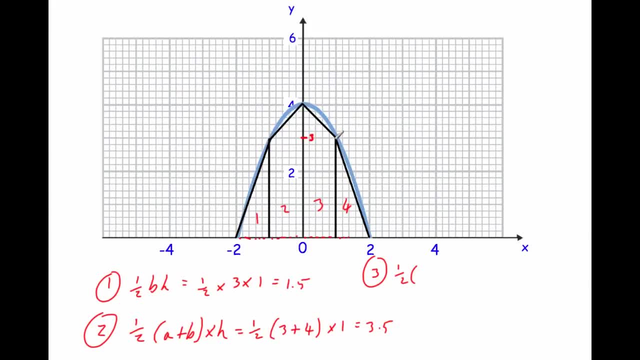 the two parallel sides added together, So this time it's four plus three, Four here and three there, So four plus three, and then times the distance between the two parallel sides, which is one, So it'll be four plus three, which is seven. Half of that 3.5 times one. again is 3.5.. And finally, region four, which is this triangle. Again we're going to do half the base. times the height, It's going to be half times the base. Again, we're looking at the base this way, So it's going to be 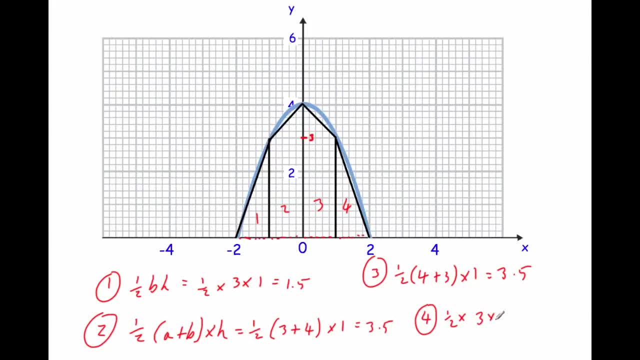 three times one. So three times one, and that gives us 1.5.. And when we add those all up together, we're going to get 1.5 plus 3.5 plus 3.5 plus 1.5. And when we add those all up, we're going to get 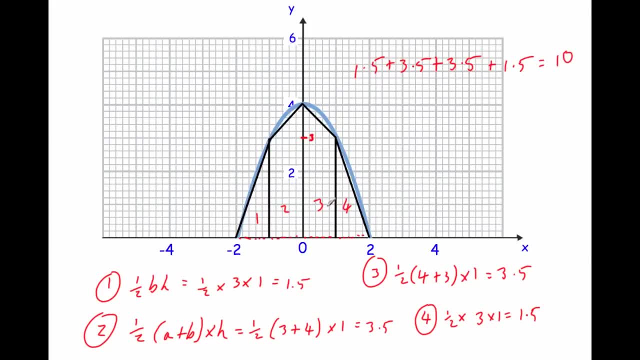 five, five and that's 10.. So the area is 10 units squared. Because there are no measurements, because this is just an x- y axis, we'll just call this 10 as the area. You'd write 10 units squared. Okay, let's have a look at example two. So example two says: below is a speed time graph of a car over: 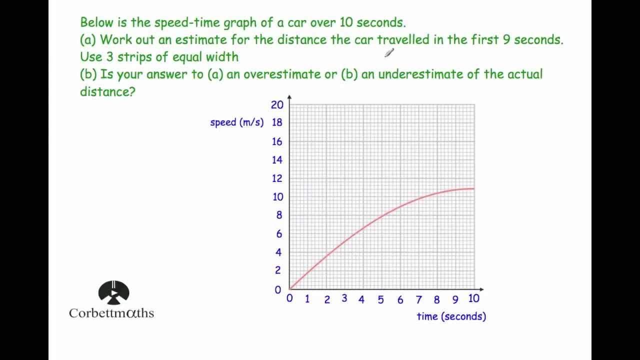 10 seconds, Part a: work out an estimate for the distance traveled by the car. in the first nine seconds I'm going to use three equal width strips, or three strips of equal width, And then we're going to answer: is the answer to a an overestimate or an underestimate of the actual distance? 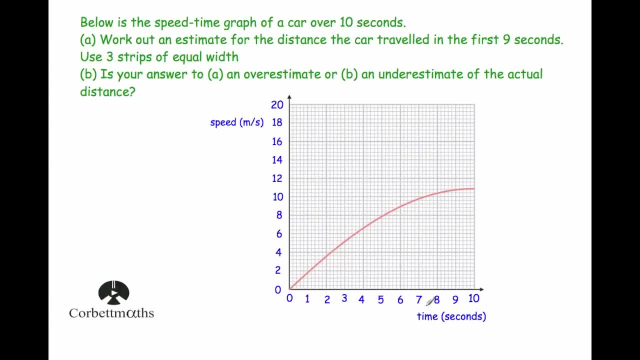 traveled. Now, one thing to note is that this is a speed time graph And if you've got a speed time graph, if you find the area underneath the curve or the, the lines that are there, that would give you the distance traveled. The reason is, if you were to find, for instance, if we had a rectangle, just say: 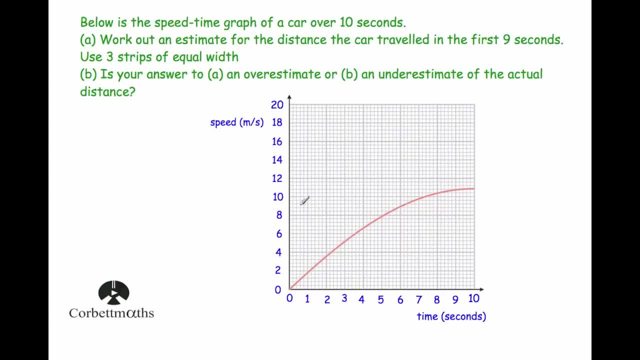 here and we were to do two times, whatever the height would be, just say 10 to get that area. We're timesing the time by the speed and just remember distance equals speed times time. So a few times together the speed and the time you're going to get the distance. So that's how the area 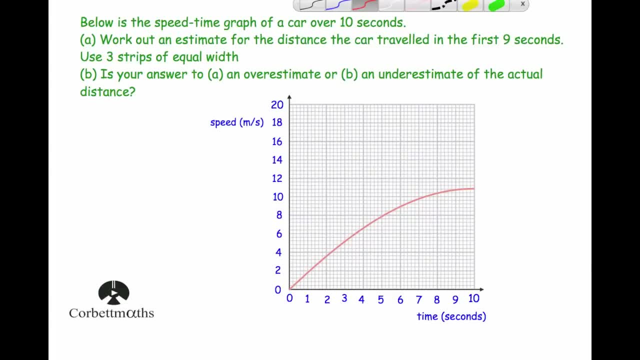 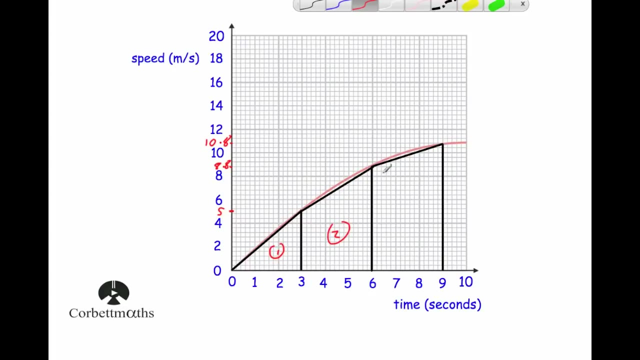 distance travels. OK, so part a, let's cut it into three equal width strips. Now the first nine seconds. Well, that means we're going to put a line every three seconds of three, six, nine to give us three regions, like so. So we've got region one, which is a triangle, region two, which is a trapezium. 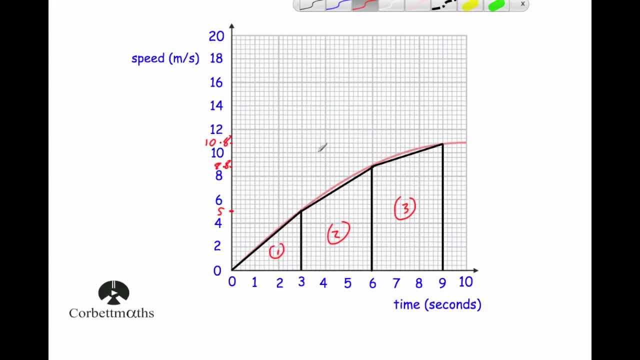 and region three, which is also a trapezium, And what I've done is I find the height of each of the lines drawn. So the line at three has a height of five. So, in other words, at three seconds the curve was at five meters per second. At six seconds it was traveling at 8.8 meters per second and at 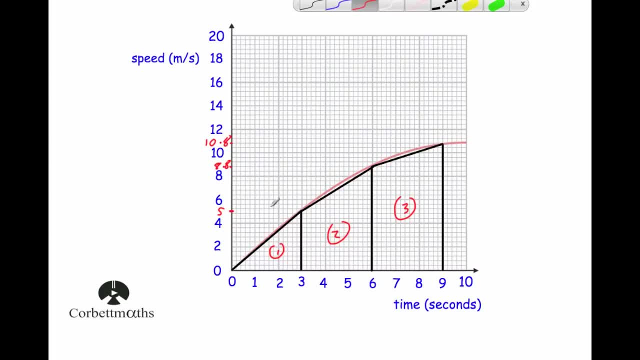 nine seconds, it was traveling at 10.8 meters per second. OK, so let's find the area of triangle one. So triangle one, half the base times the height Again, because the trapezia are this- are sort of sidewards, that the height or the distance between them will be the three. So again, I'm going to 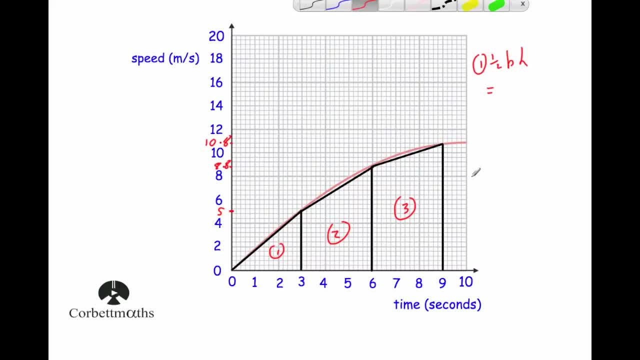 consider this being the height of the triangle, So I'm sort of looking at each one sidewards. So a half Times the base. Well, the base is equal to five And the height of it is three. So five times three is 15 and half of that is 7.5.. So this one here is 7.5 meters because if you do meters per second, 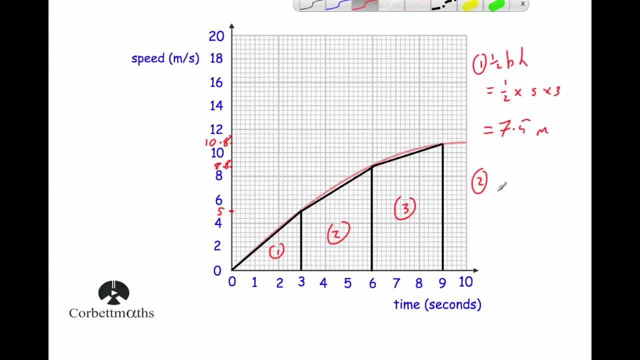 times seconds. it's going to be in meters. OK, trapezium number two. So it's going to be a half bracket, a plus b times the height, So half of the two parallel sides. Well, it's five and 8.8.. So five. 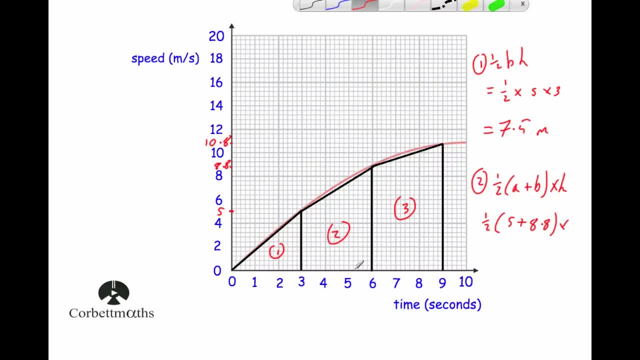 plus a plus b times the height, So half of the two parallel sides. Well, it's five and 8.8.. So five plus 8.8.. And we're going to be timesing that by the distance between them, which is three, And when we do. 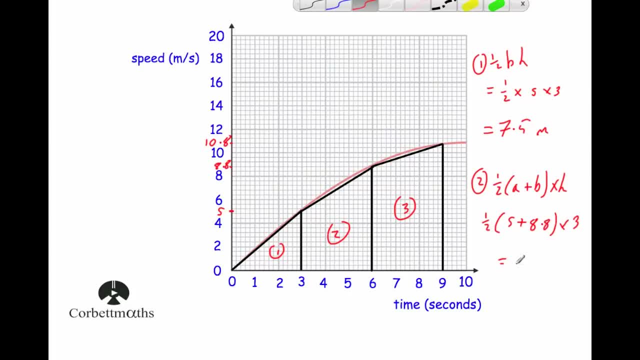 that we're going to do five point five, or five plus 8.8, which will be equal to 13.8.. And then we're going to times that by three and half. it So 13.8.. I'll divide it by two first of all, And then I'll 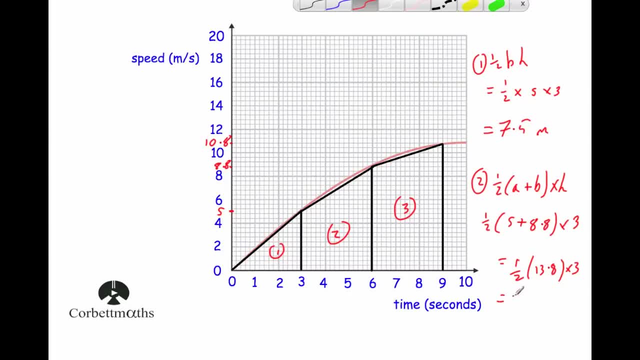 times it by three And I've got 20.7.. So that's 20.7 meters. So in this region the car or between three seconds and six seconds. the car traveled approximately 20.7 seconds. Remember, it's an approximation because, because the line doesn't quite sort of cover the whole area of the, of the 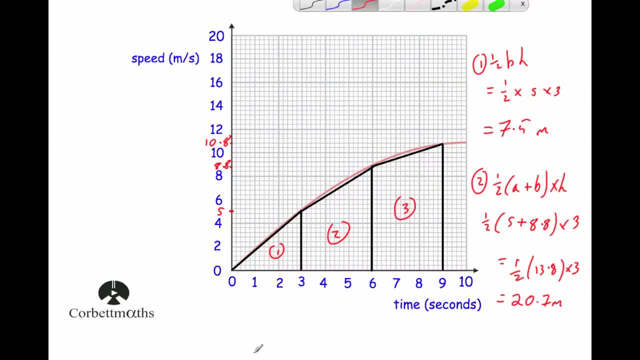 curve. OK, We've got this little bit here, that we haven't found the area of. OK, I'm three, The last trapezium, which is this one. So again, it's given by the formula half the two parallel sides added. 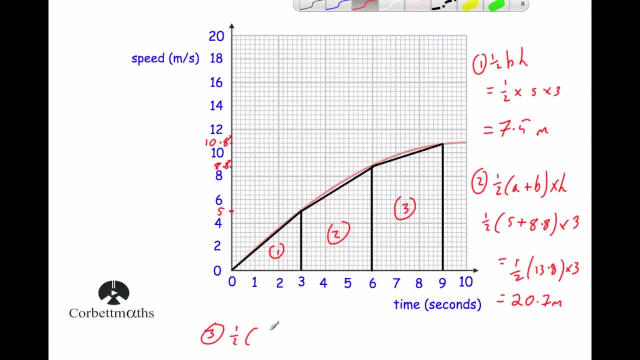 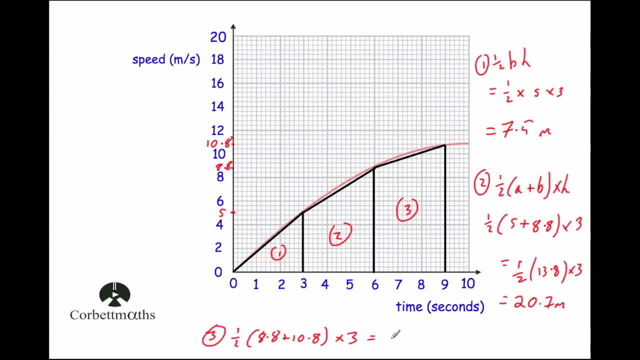 together. So that's 8.8 plus 10.8.. So 8.8 plus 10.8.. And we're going to times that by the distance between them, which is three, And when we do that we get an answer of 29.4 meters. So to get the 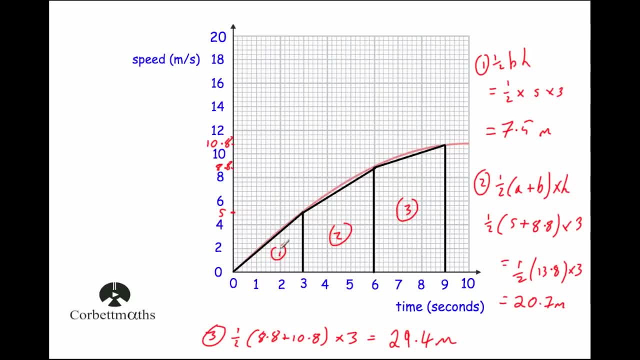 total distance traveled by the car. we just need to work out, or an approximation for the total distance worked out, travel by the car. We're going to add together the area of triangle one, of trapezium two and of trapezium three And we'll see what we get for the total area. So we're going. 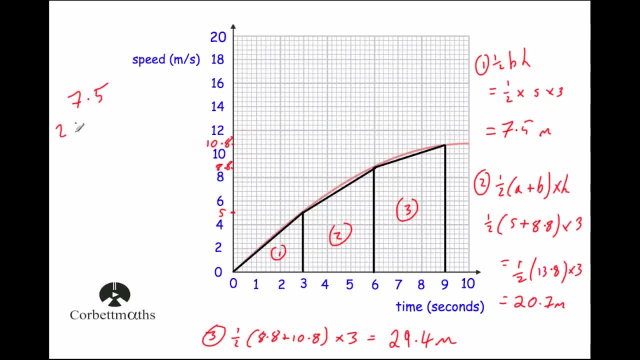 to do seven point five plus twenty point seven plus twenty nine point four. When we add those two together, we get 57.6 meters, And that's the total distance traveled by the car, or an approximation to it. Remember, it's not quite right. In fact this would be an underestimate. 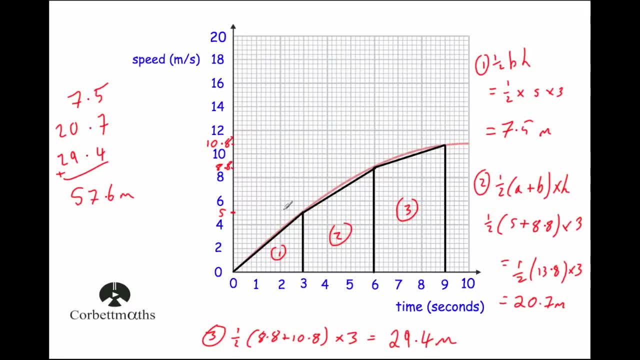 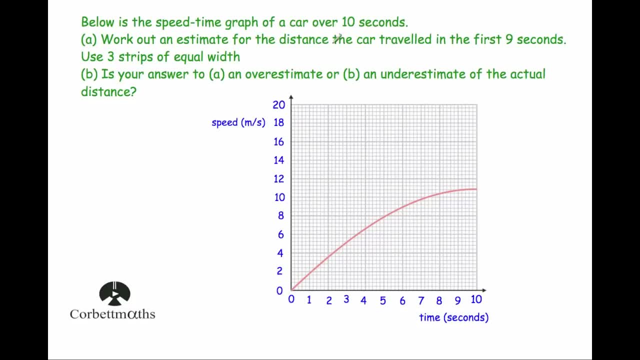 because the actual red line is just slightly above our ships. OK, So if we go back to the question now, as you can see, the part A says: work out an estimate for the distance the car traveled in the first nine seconds. So, as we've worked out, that is 57.6 meters. So 57.6 meters And part B is your. 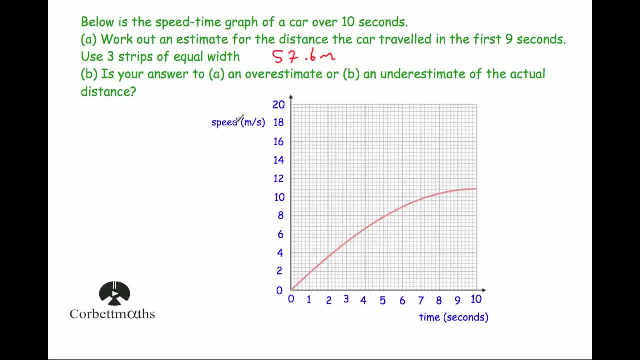 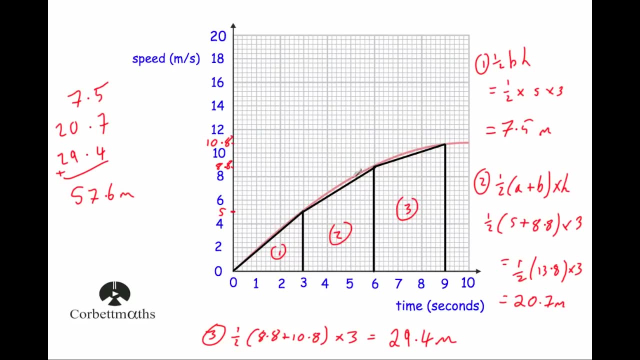 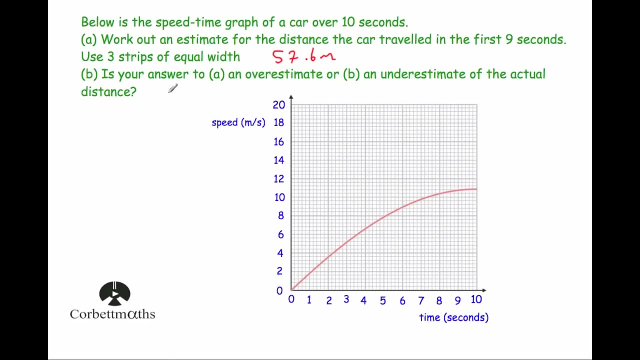 answer to A: An overestimate or an underestimate of the actual distance traveled. We've kind of already answered this. As you can see the triangle, the trapezium and the trapezium all underneath that red line. So our area is just slightly under the actual area. So our answer is an underestimate. So part B it. 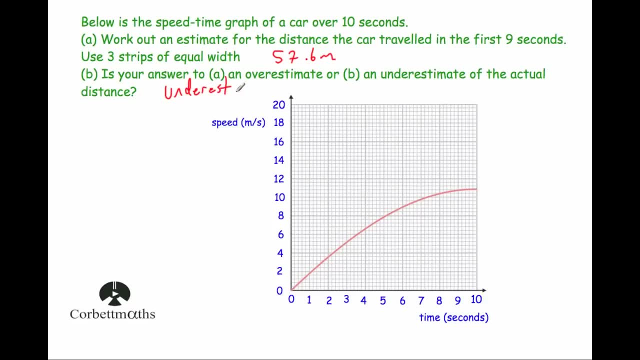 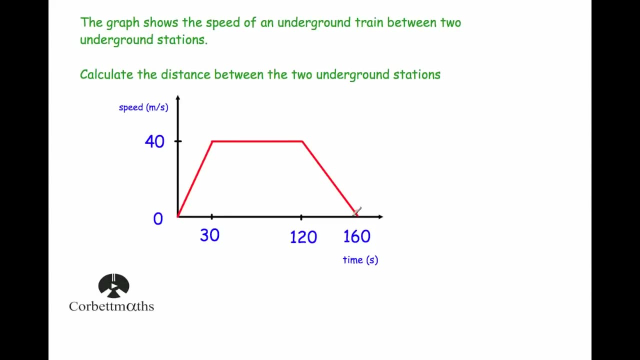 is an underestimate. OK, Now, sometimes the questions that we're given will have straight lines which can be a little bit nicer, where we're not having a lot of time to answer them. But we're going to do that. We're going to have to estimate things, OK. So this question says: the graph shows the speed of an. 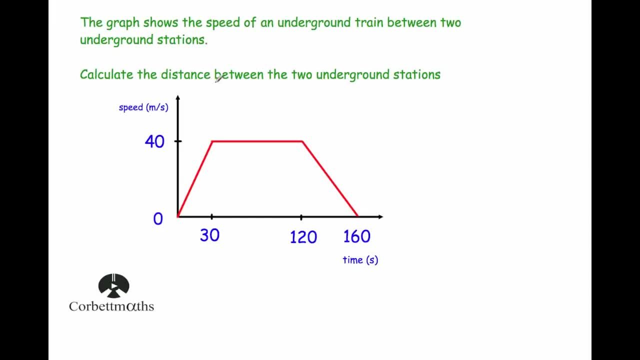 underground train between two underground stations. Calculate the distance between the two underground stations. So here we've got the speed, and it sets off from zero meters per second And after 30 seconds reaches speed of 40 meters per second. It travels at that speed until a total. 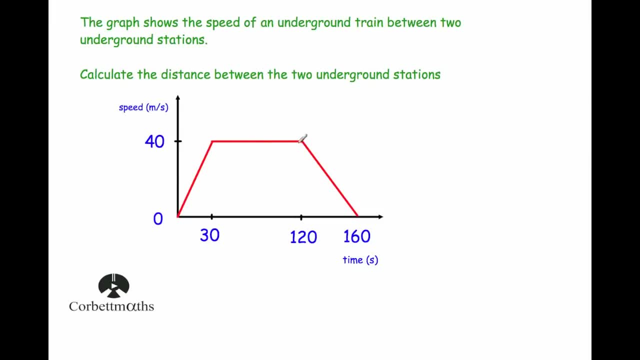 time of 120 seconds has gone, So for another 90 seconds And then over the last 40 seconds it slows back down to rest. OK, So what we're going to do is we're going to split the distance between the two underground stations. Calculate this up into shapes. We could do it as one trapezium. I don't. 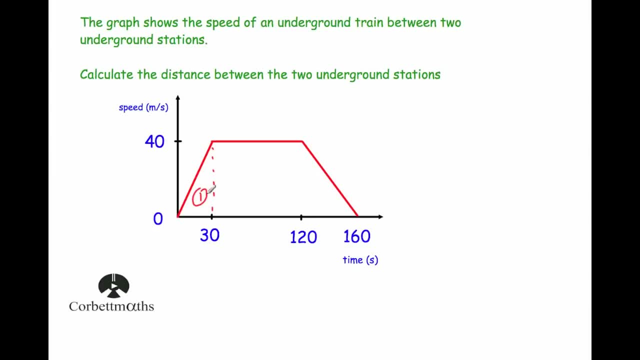 know why, but I tend to just cut it up into triangles and rectangles. So one, two and three. OK, So to work out the areas of these, I'm going to do half the base times the height for one. So half the base times the height, So it's going to be a half times the base. Again, I'm going to consider. 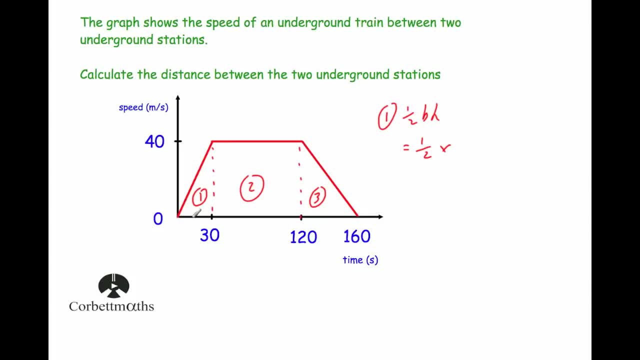 this to be the. actually it wouldn't really matter because I've got no trapezium so it doesn't really matter. So I'm going to do 30 times 40. And half it, So that's going to give us 600 meters for the region, one For the next part of the. 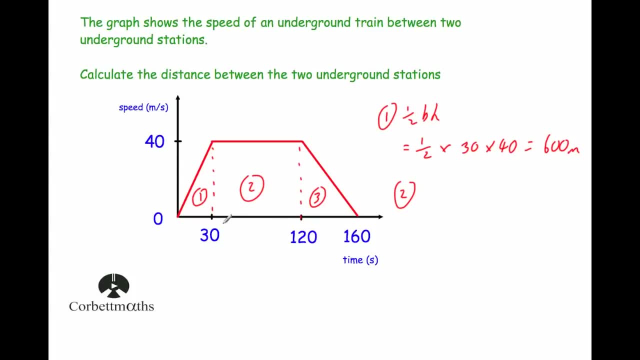 journey from 30 seconds to 90 seconds. Well, that means, sorry, from 30 seconds to 120 seconds. Well, that means it's 90 seconds in total there for that section of the journey, And so we're going to do length times width, So it's going to be 90 times 40. And that will give us three thousand. 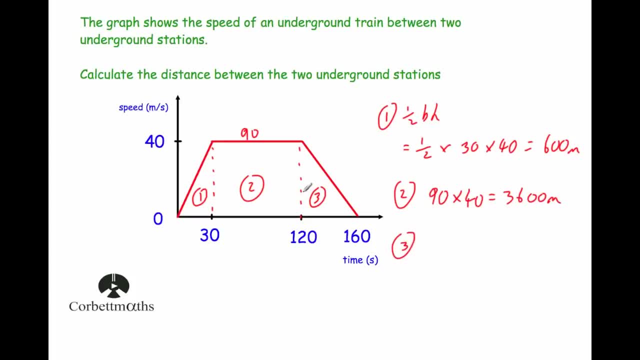 six hundred meters, And our last section of the journey is this triangle And it's going to be obviously a half the base times the height, So half the base. Well, the base from 120 to 160 is 40. So half of 40 times the height, which is 40, which will give us 800 meters. And then we just need to 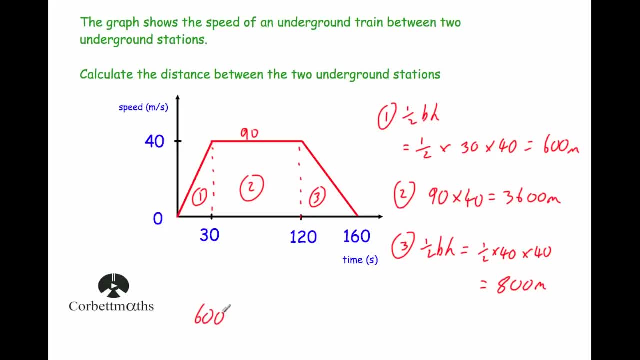 add them up to get the total distance travelled, So it's going to be 600 plus three thousand six hundred plus eight hundred, which is going to give us four thousand two hundred five thousand meters. So five thousand meters or five kilometers. OK, And the last example. So our last example. This time, what we've got is we've got a speed times. 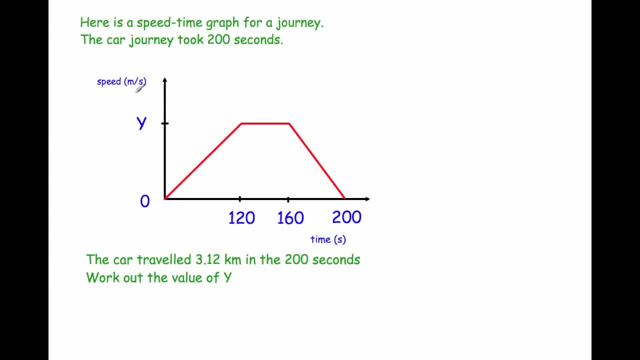 graph, Speed time graph for our journey. But rather than tell us to tell us the speed, we've got the speed given as y And it tells us that the car journey lasts 200 seconds. Well, we can see that from the graph And it tells us the total distance travelled. So the total distance travelled is 3.12. 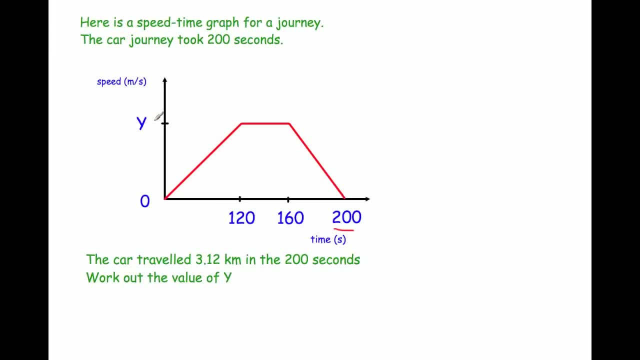 kilometers And we've got to work out the value of y. So what we're going to do again is I'm going to split this up in two: The triangles and the rectangles. So we've got one, two and three, And we're going to find the areas of these three and get them in terms. 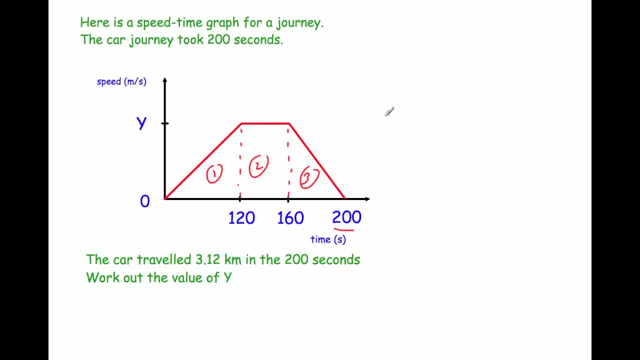 of y to begin with. So before we begin, also, we know the distance is 3.12 kilometers. I'm going to change that into meters as three thousand one hundred and twenty meters, just because it's the speeds given in meters per second. OK, Firstly, region one. Well, again, it's a triangle.